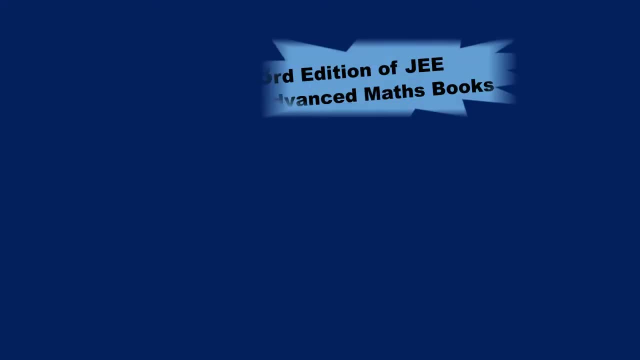 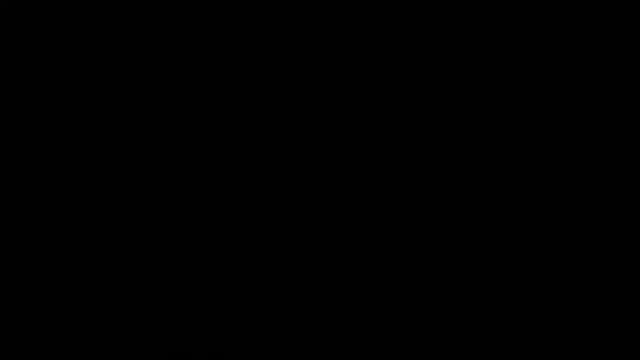 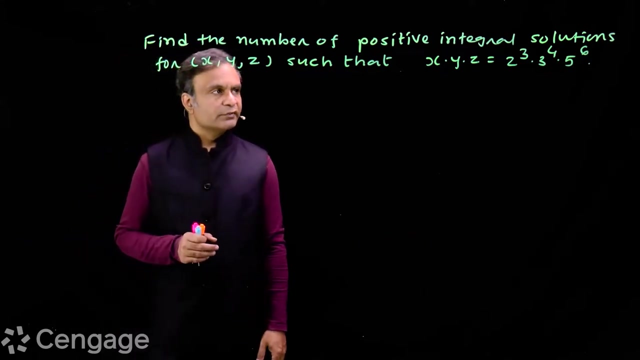 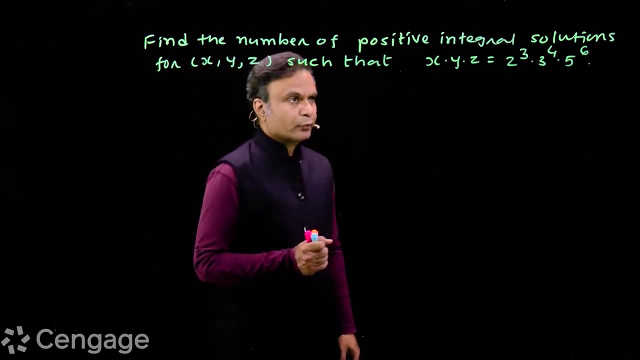 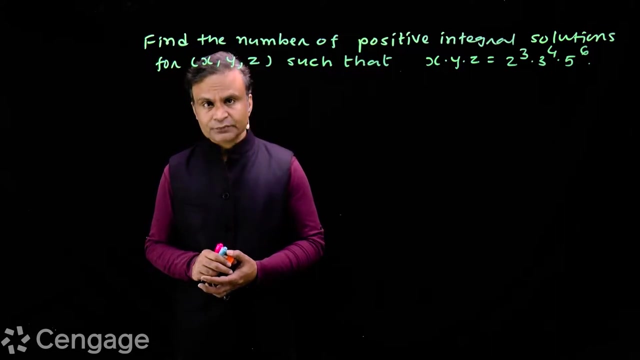 Now, here we have a very interesting application of this concept. The question is: find the number of positive integral solutions for triplet x, y, z such that product x, y, z is equal to 2 cube multiplied by 3 power 4, multiplied by 5 power 6.. Here we have a 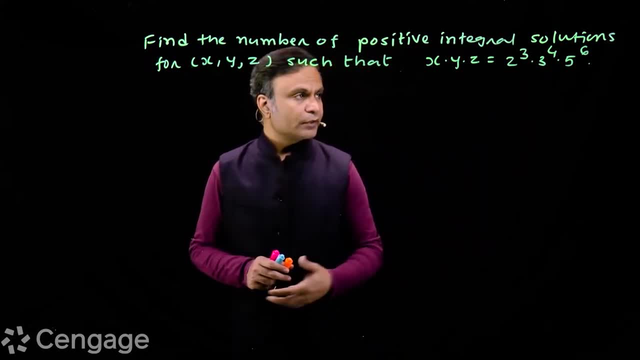 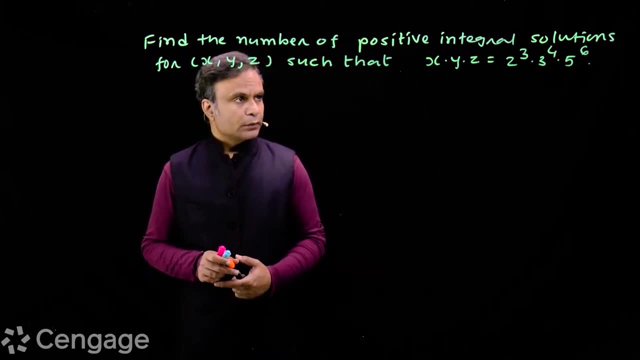 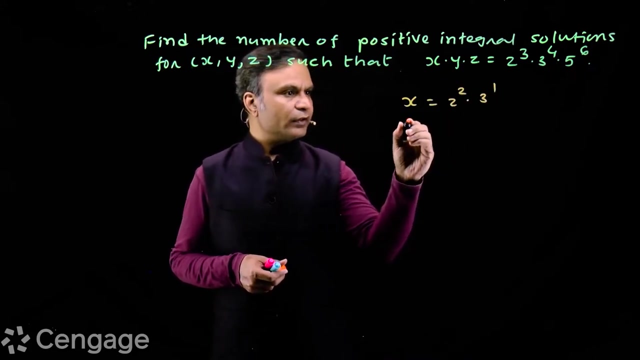 value in the form of prime factorization. Here values 2, 3 and 5 are prime numbers. Now what do you mean by positive integral solutions of this equation We may have: x is equal to 2 square multiplied by 3 power 1, and y is equal to 2 multiplied by 3 square. 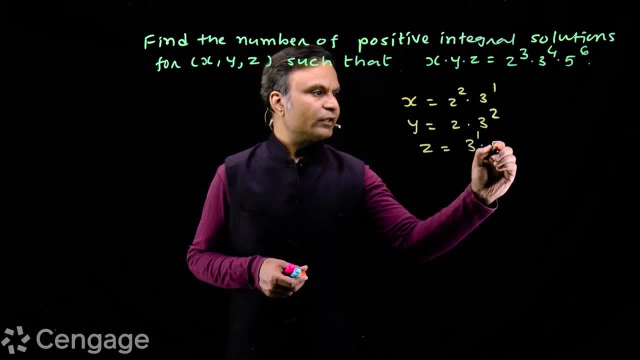 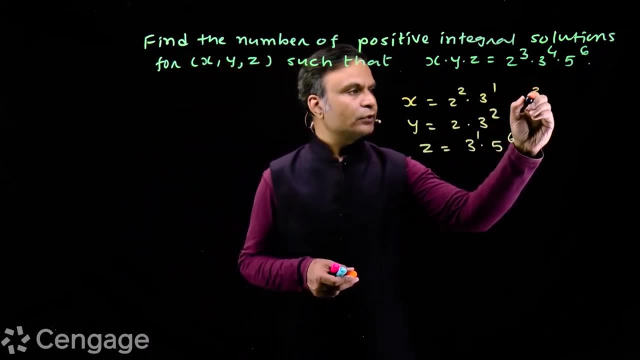 and z is equal to 3 power 1 multiplied by 5, power 6.. So this is one of the solutions We may have: x is equal to 3 square multiplied by 5 square y as 2 multiplied by 3 multiplied. 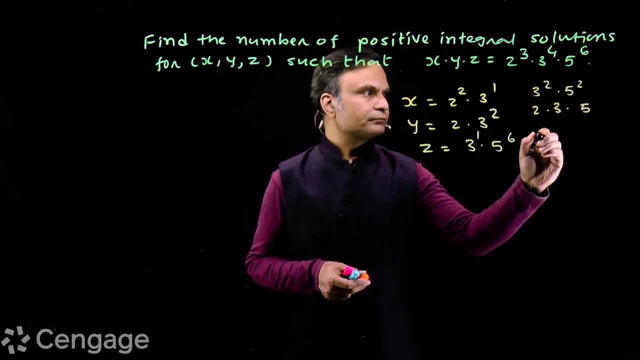 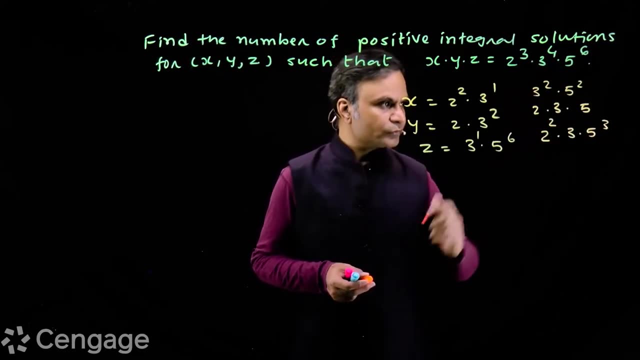 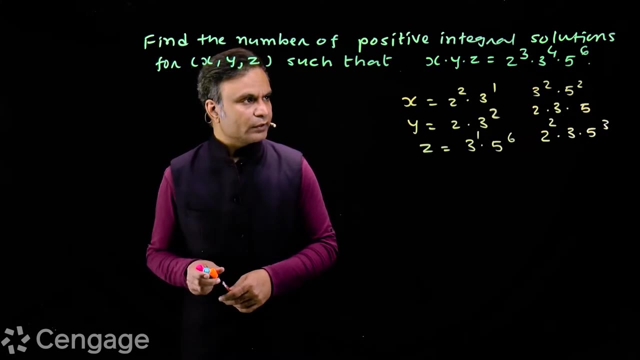 by 5 and z as 2 square. So we have: x is equal to 2 square multiplied by 3, multiplied by 5 cube. This is another solution. We have so many solutions. Now, what exactly we are doing? We are actually. 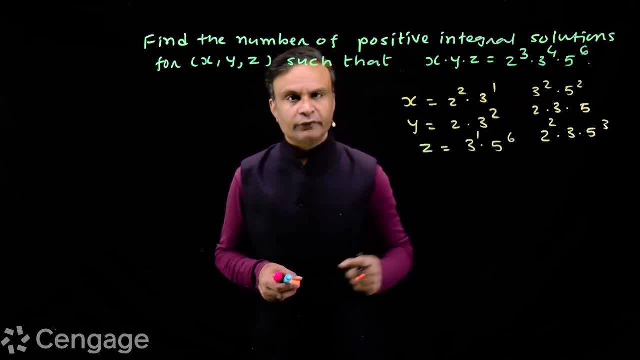 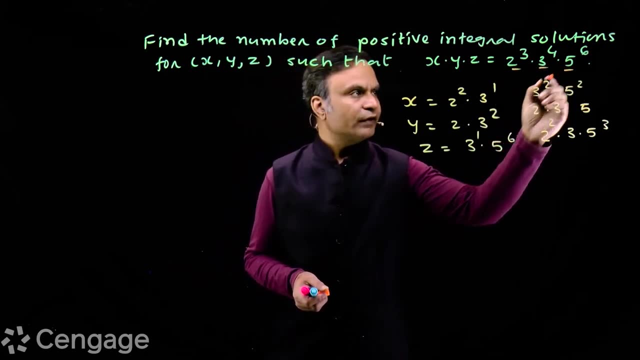 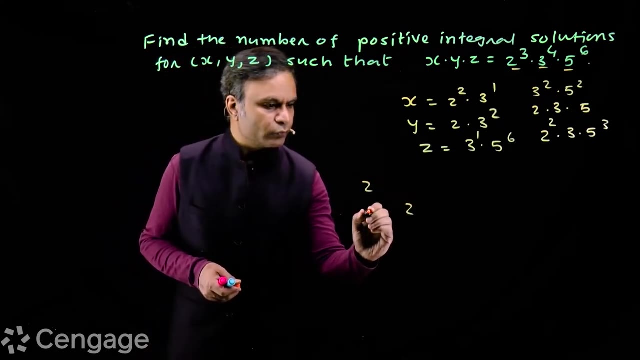 distributing prime factors 2,, 3 and 5.. We have prime factor 2 three times, We have prime factor 3 four times and prime factor 5 six times. So we first write this: prime factors In groups. we have 2,, 2, 2.. This is one group of identical objects. 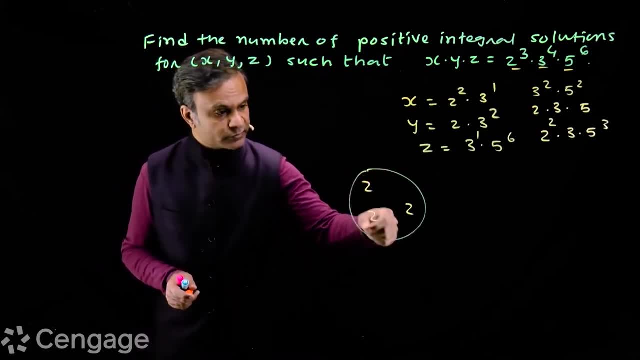 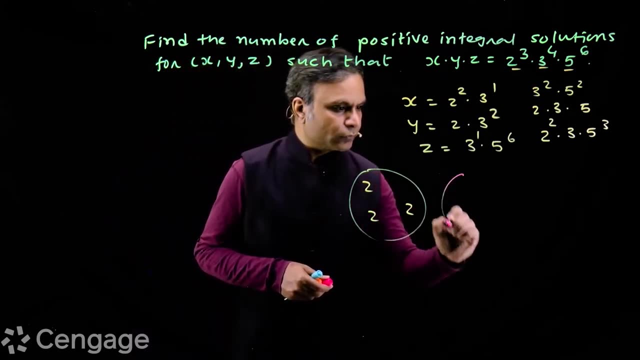 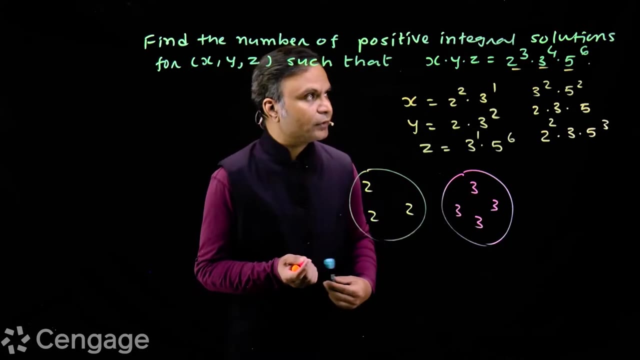 Here I gave you an idea. Here these three objects are identical, of one kind. Then we have 4 identical objects of other kind, 3,, 3,, 3, 3, and then we have 6 objects of third. 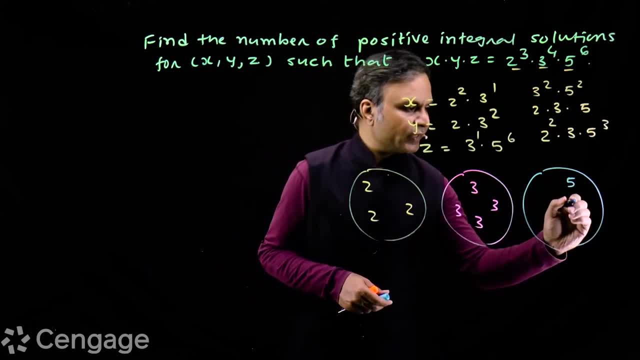 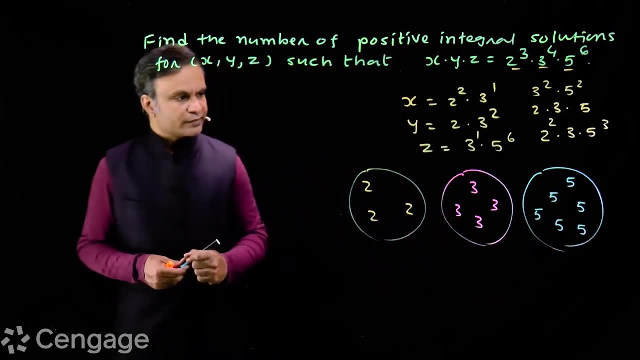 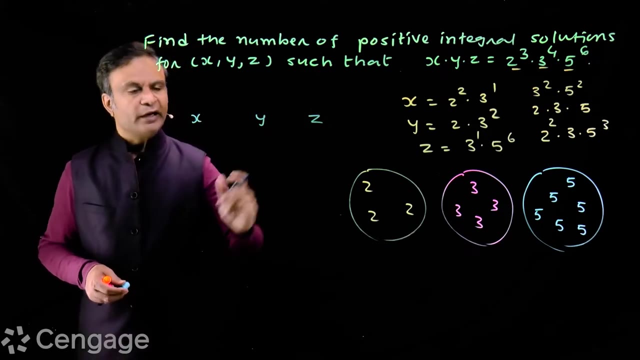 kind. We have 6 identical objects of third kind, that is, 5,, 5,, 5,, 5,, 5, 5.. Now what actually we are doing? We are distributing these objects into three boxes, namely x, y and z. I have made three boxes here, named x, y and z, And 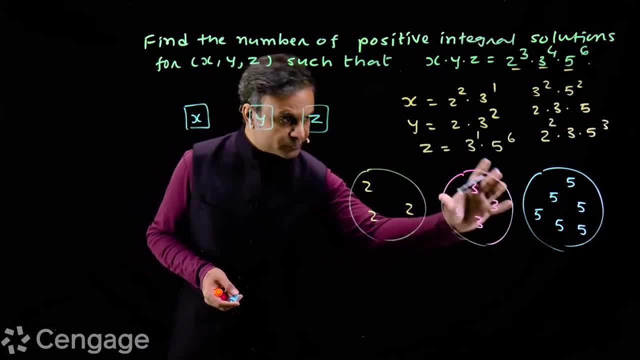 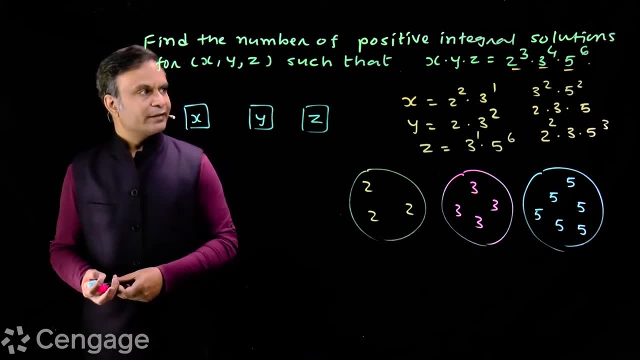 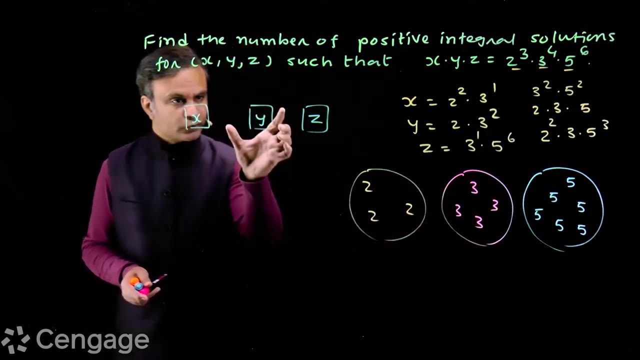 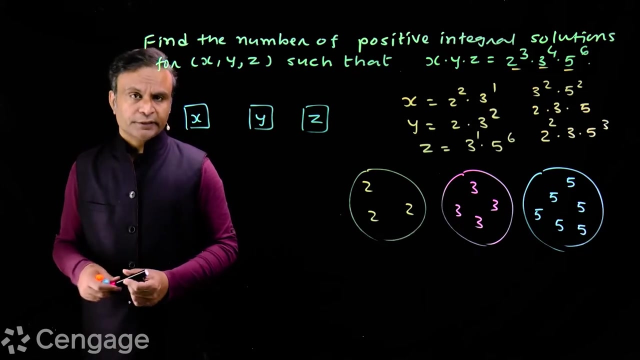 what we are doing. We are distributing these objects in these boxes. Then we can say: number of positive integral solutions is equal to number of ways we can distribute these objects into these three boxes with name x, y and z. So how will we solve? Here we have these three identical objects. How we distribute. 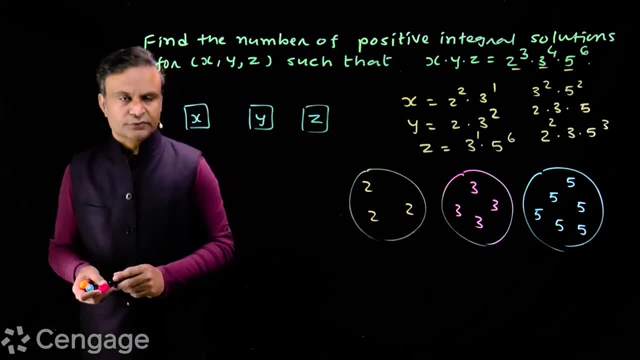 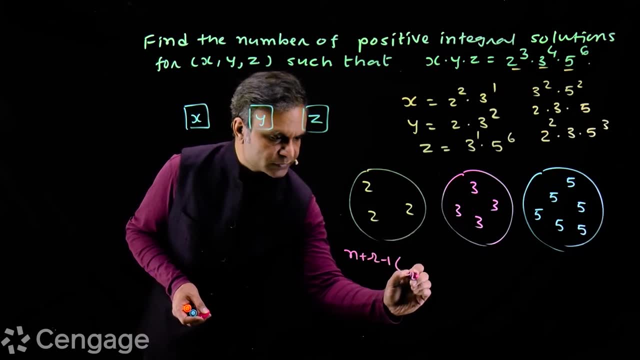 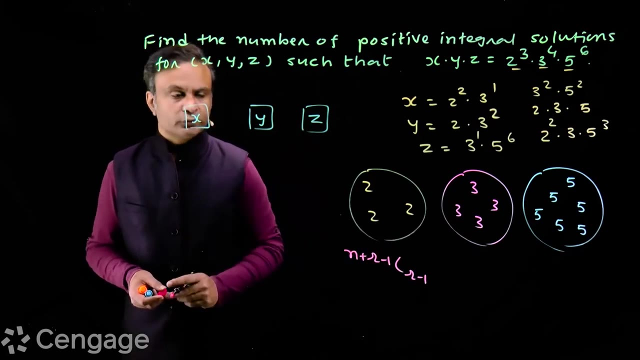 these three identical objects into three distinct boxes. We use the formula n plus r minus 1, c, r minus 1.. Here number of objects n is equal to 3, number of boxes r is equal to 3.. So we have number of ways of distribution of these three prime factors into these three. 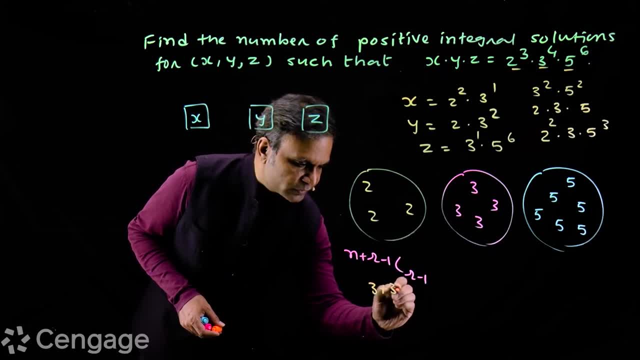 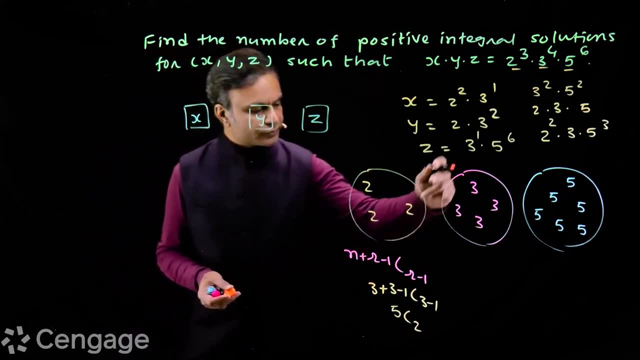 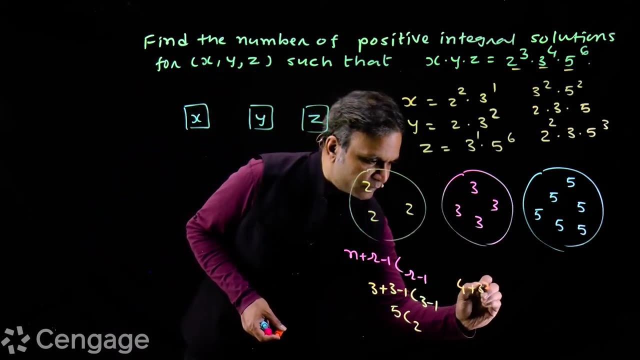 boxes, distinct boxes as 3 plus 3 minus 1 c 3 minus 1 and this is 5 c 2. Now we distribute this. four identical objects We can distribute in 4 plus 3 minus 1, so 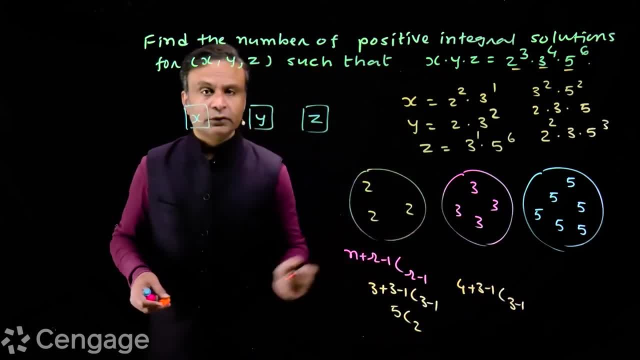 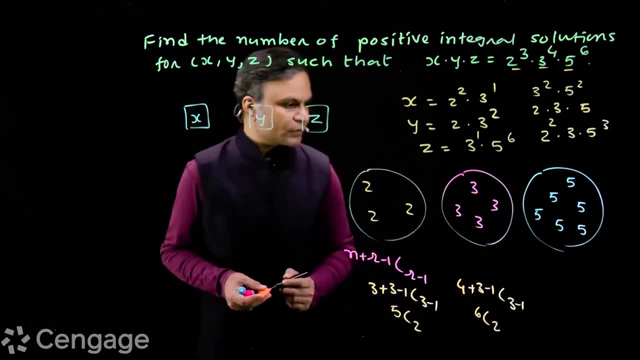 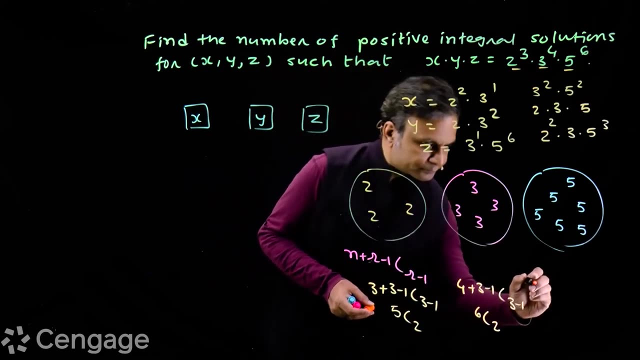 minus 1 c, 3 minus 1. here value of n is equal to 4.. So this is equal to 7 minus 1, 6, 6 c 2, and we can distribute the 6 identical objects into this: 3 distinct boxes in 6 plus 3. 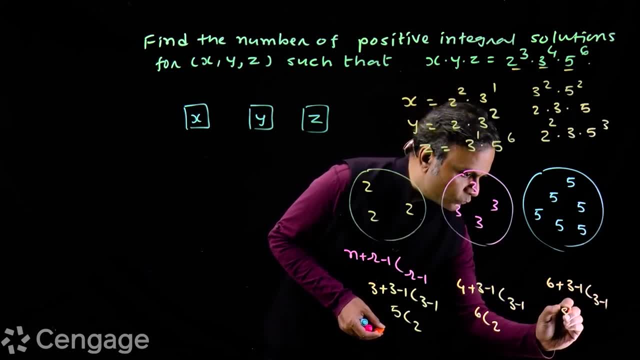 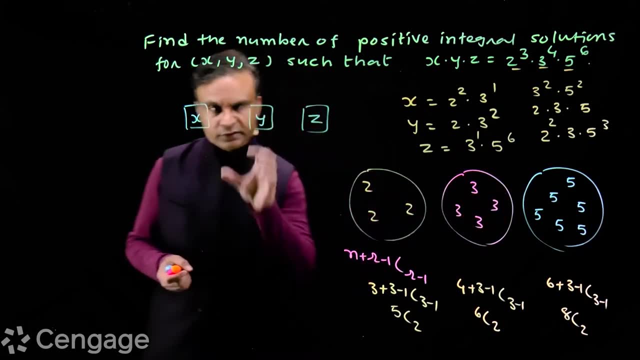 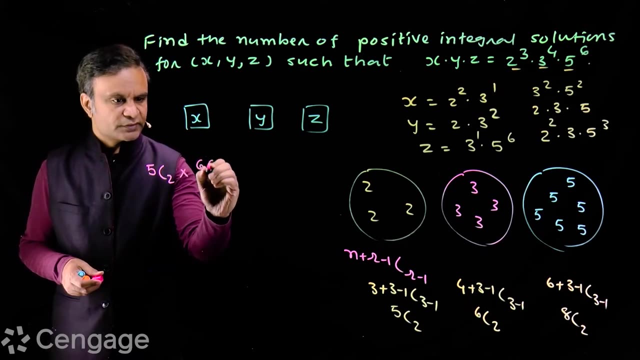 minus 1 c 3 minus 1 and this is equal to 8 c 2.. So total number of ways of distribution of all this prime factors into this 3 distinct boxes as 5 c 2 multiply by 6 c 2 multiply. 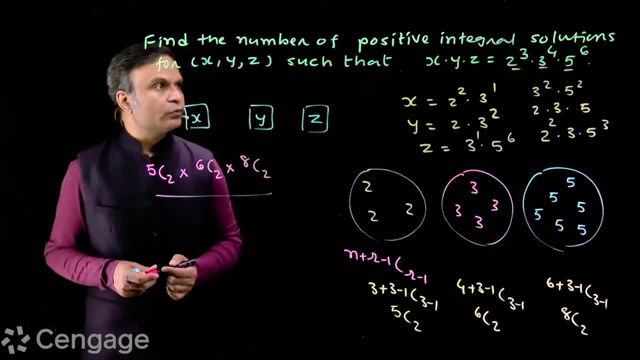 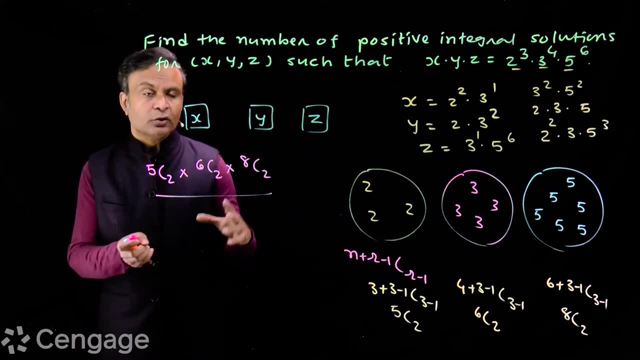 by 8, c, 2. So this is equal to number of positive integral solutions of this equation. So see here, with this concept- distribution of identical objects concept- we have solved this equation. Now it may happen that x is getting none.